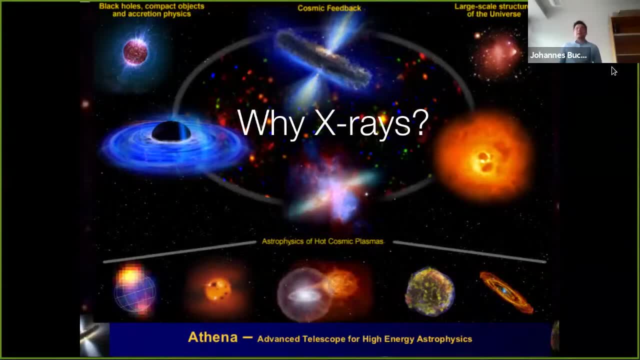 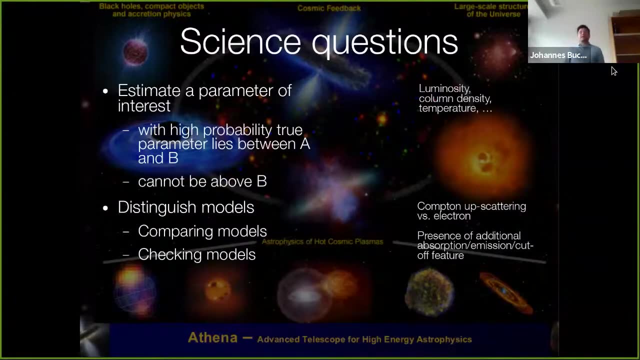 And they are very interesting systems to study And X-rays allows us to do that. Just in general, the science questions we typically have here. I divided them in two categories, For example. you might be interested in some parameter of interest, for example. 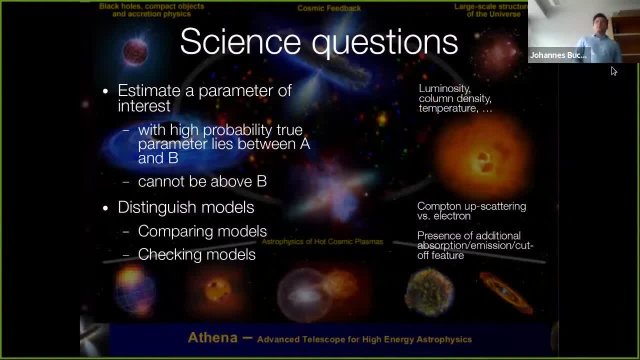 aluminum And you want to make a statement that, with high probability, the true value out there in the universe lies between A and B. Or you might want to say, oh, it cannot be above B, Otherwise the data would be very different. And the second type of science question we have is: we want to 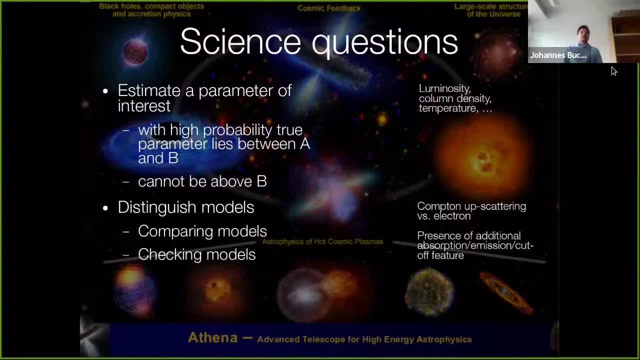 distinguish different processes, or, for example, Compton-Op scattering versus, or something like that. Or we want to test for additional absorption, emission or cutoff features, something like that. So that would be comparing models, And another aspect of this is checking whether one particular 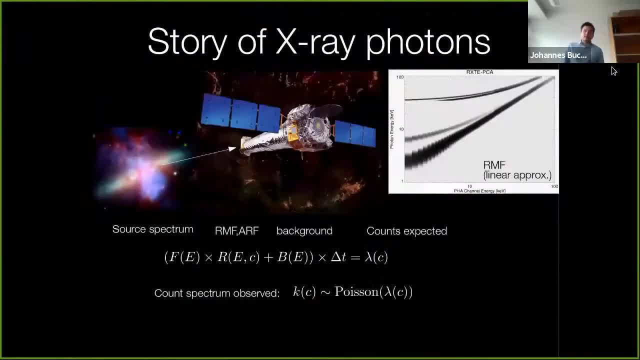 model can actually explain the data. Here I just want to give a bit of a brief story of how we tell ourselves the observations are done, And I'll talk in particular about X-ray spectra from a point source, But many of these concepts can be. 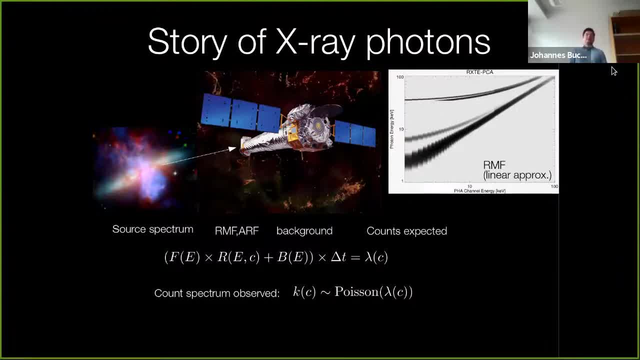 transferred to other data like timing and imaging. So on the left you have your astrophysical source With its source spectrum. the X-ray photons enter the mirror modules of the telescope, are twice reflected and focused on the detector, where they are transformed into an electron cloud. 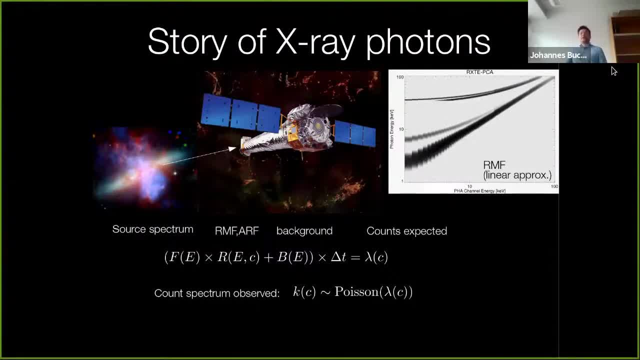 and become counts in energy channels, And we can model this whole process And we can do this whole procedure by projecting through a response matrix. One is an example shown on the top right here And you see it's not a diagonal matrix, So we 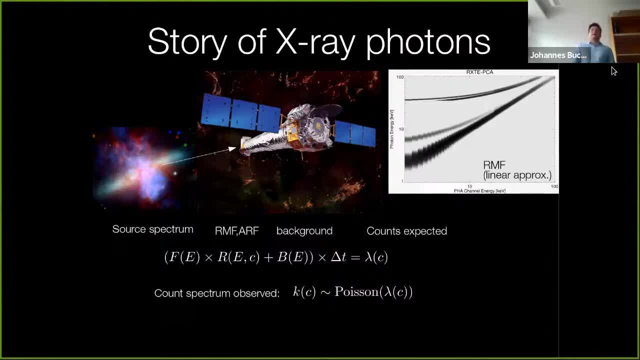 cannot invert this process. to infer the source spectrum We have to forward fold and to estimate the counts expected on the detector. So if we do this linear approximation, basically you assume some source spectrum, You assume you know your instrument, You assume you're. 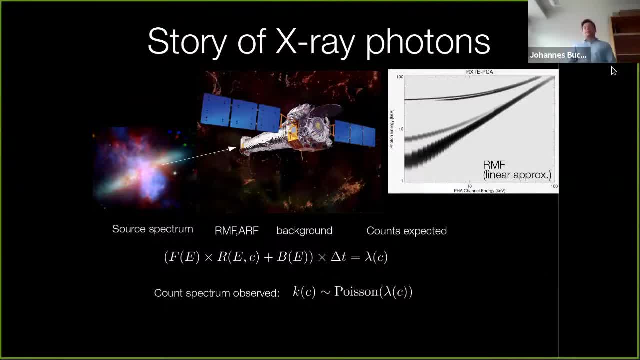 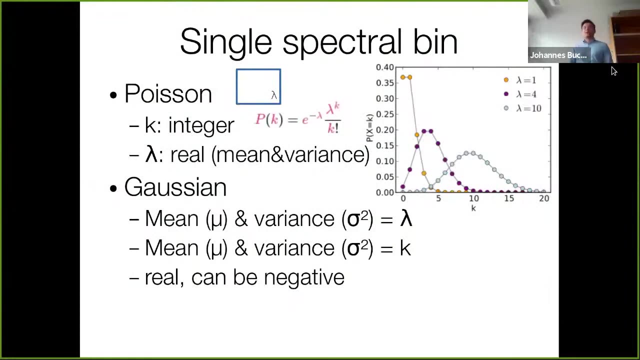 additionally have some background emission coming in And you can simulate what you would expect, how many counts you would get, And then you can make a Poisson realization of that to compare to your actual data. Just to remind you about count data, here is the Poisson distribution formula. 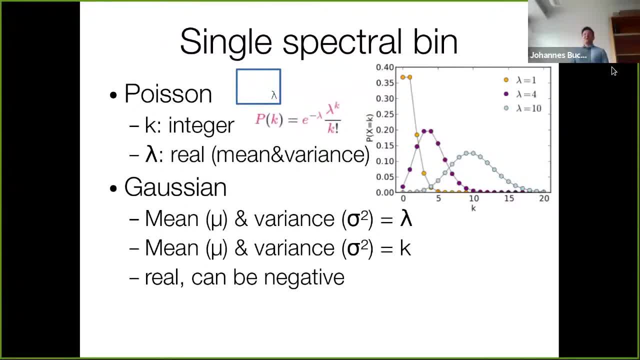 and plotted on the right. The counts are integers and they cannot be negative. So we can do this by looking at the dock And you see from the distribution that it's not a symmetric distribution. So if you use gaussians they will lead to biases. 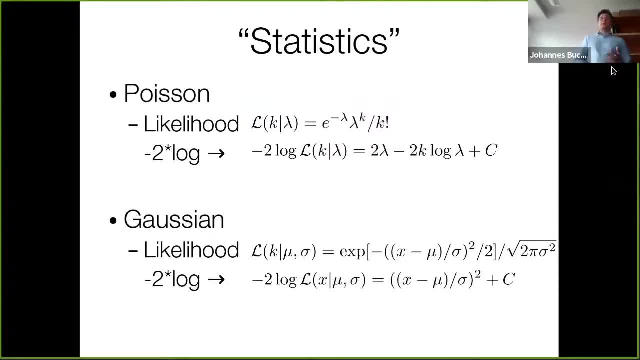 in the low counter regime for sure. I remind you also that if you take this Poisson likelihood that I just showed you and you apply this trick of taking the logarithm and multiplying by minus two, you get this formula here, which is known as Cstat, or cache statistics. 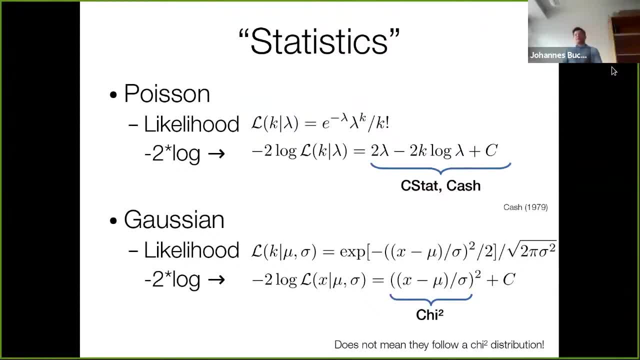 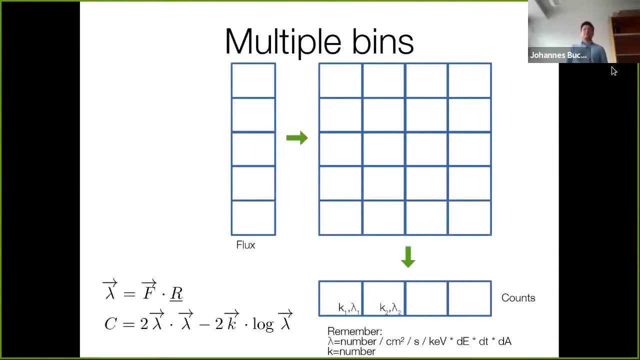 depending on what constants you drop. If you do the same with the Gaussian likelihood, you get what's called chi-square. This doesn't mean anything except saying, oh, we assume a Poisson data process or a Gaussian data process. If you have multiple bins, you project this through. 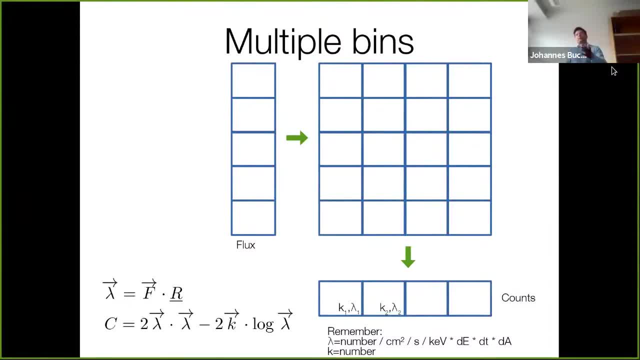 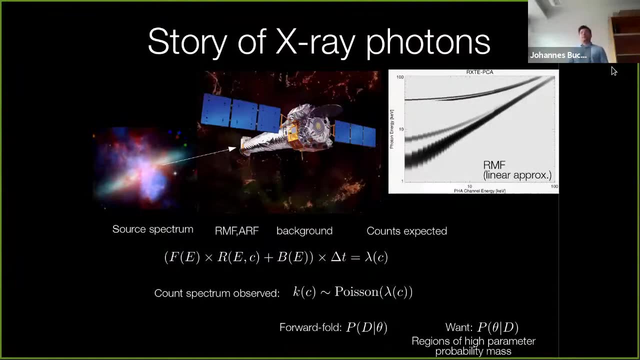 As I said, your flux spectrum, you project it through your response and you get the number of counts you expect in each energy channel. You sum up your statistic and that gives you your likelihood. So we've established this forward folding that gives you the probability to produce some data. 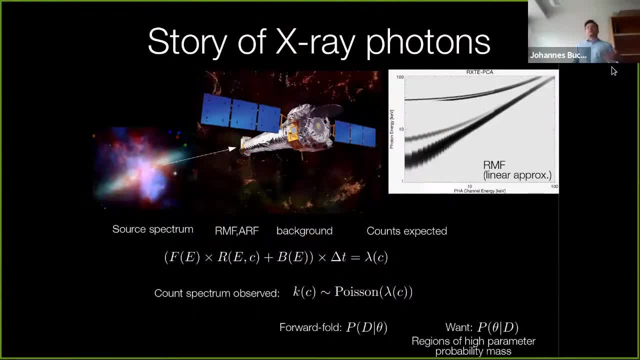 assuming all of this process, assuming a source spectrum instrument model and so on, And that we will casually call the likelihood, But what we actually want is the probability distribution of the source spectrum parameters. So we want the probability distribution over the parameter space, not over the data space. 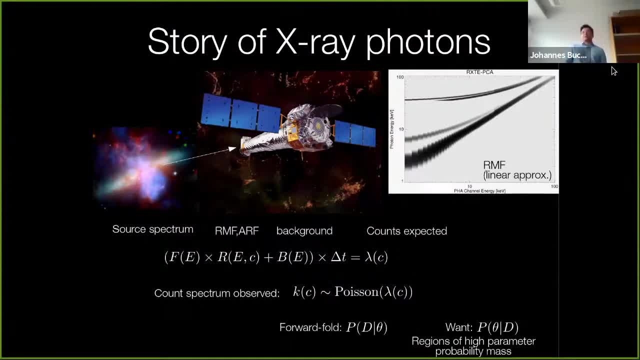 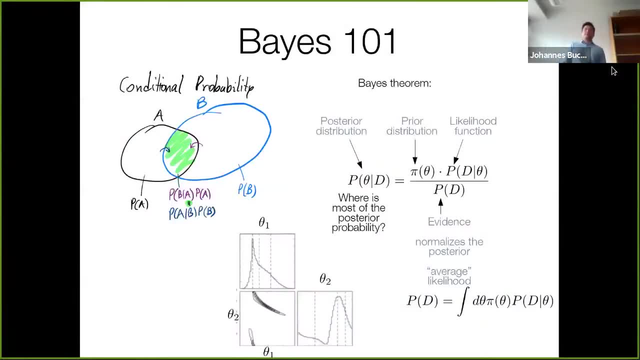 And we want to identify those regions and those parameters which have high probability. And nobody knows how to do this from scratch. but we know the next big thing, which is Bayesian inference, And I'm sure many of you have, or most of you have, heard about it. 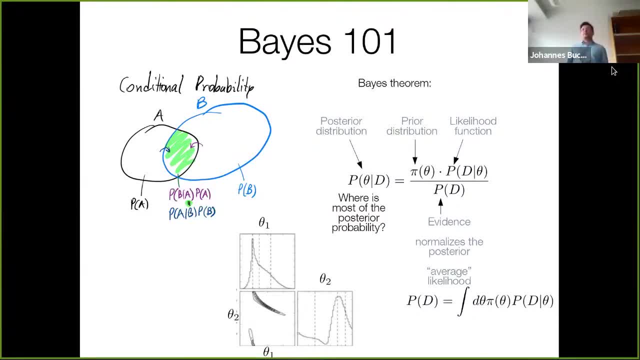 I'll just keep it brief. Basically, the idea is to start with the probability distribution, called the prior distribution. So that's already a probability distribution over the parameter And you update it with the likelihood function, which is not a probability distribution over the parameters. 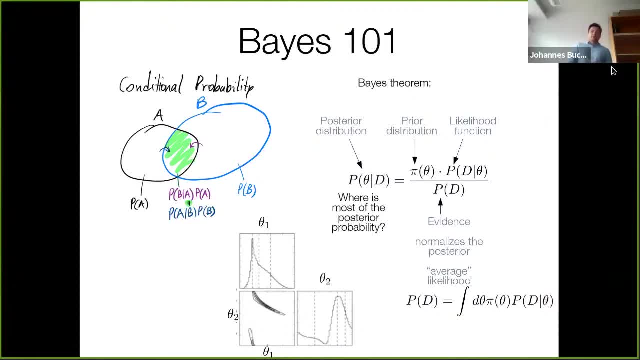 You update it and on the left you get the posterior distribution And you see here on the bottom left an example of such a probability distribution And you look at where most of the probability is, and that allows you to answer some interesting science questions. 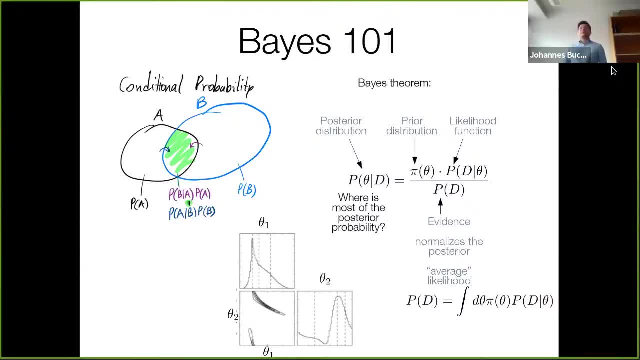 The term on the bottom right in this equation is called the evidence that normalizes the posterior. It's sort of the average likelihood over the parameter space And it can be used for model comparison that I will get to later, So you can do this. 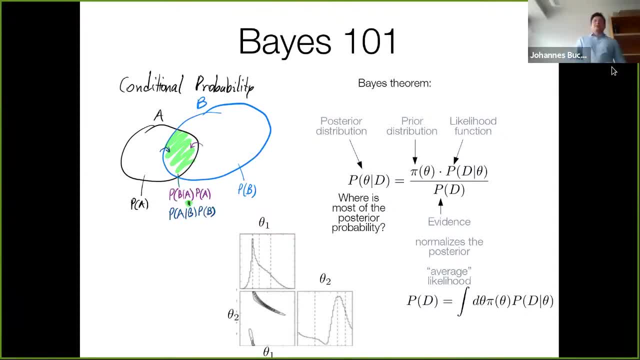 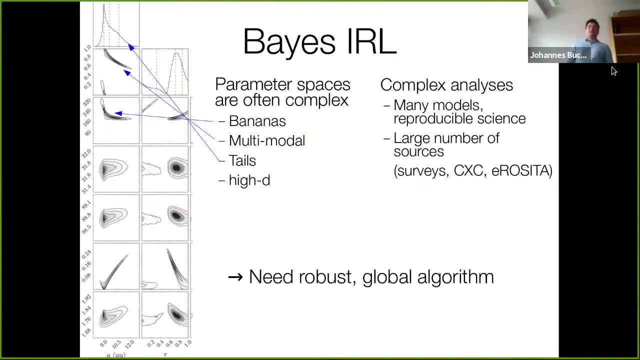 You can make grids in your parameters and you can do Bayesian inference, and everything's great. Except in real life it's a little bit more complicated. So parameter spaces like the ones shown here on the left can have these weird banana shapes where they have multiple peaks. 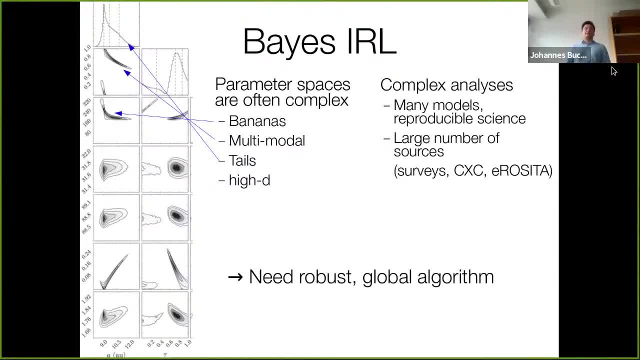 They can have odd tails, and that's important if you want to put 99% limits on something And they can be high dimensional, by which I mean you have five, 10,, 20 parameters that you want to constrain And, at the same time, 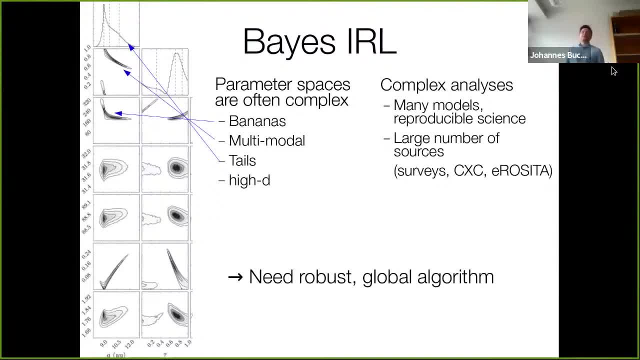 we're getting into an era where we have many sources, large number of sources from surveys, from the X-ray archives, And even if you don't have many sources that you want to analyze, you might have one particular source but many models that you want to contrast. 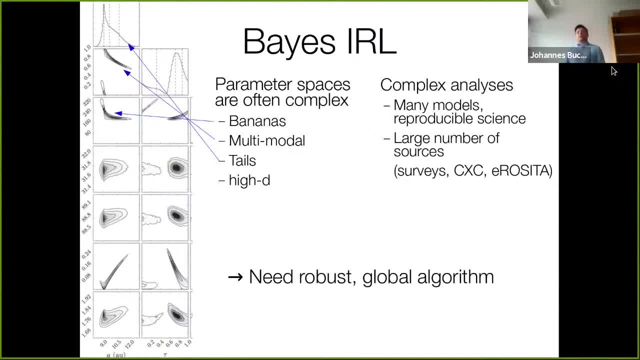 And if you want to do this in reproducible science, you want to use some robust algorithm that deals with these complications that I mentioned. So some global algorithm that allows you to automate this process- And here I'll be talking about nested sampling- which does address these problems. 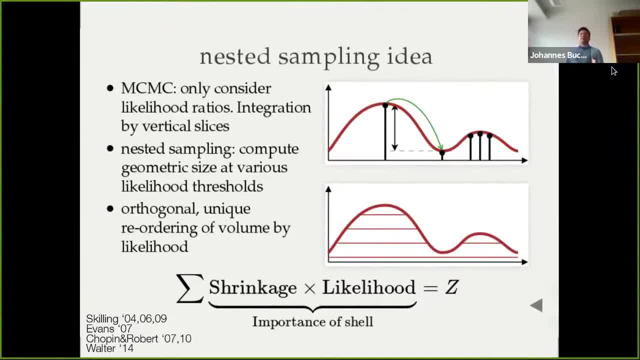 And if you're familiar with Markov Chain, Monte Carlo and CMC, it basically jumps around in this parameter space and visits, Sort of gives you the probability distribution. So you basically build a histogram in these vertical slices. but nested sampling works sort of the other way around. 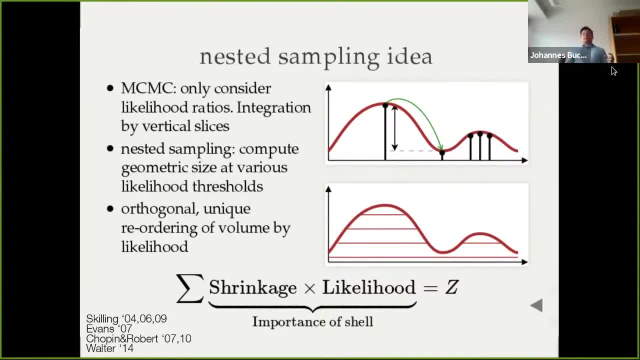 It makes horizontal slices. So you try in each iteration to build one of these Lebesgue slices and compute the height of the slice, which is the likelihood, and the width or the volume of this accessible parameter space And at the same time, And the integration over these slices is then the integral. 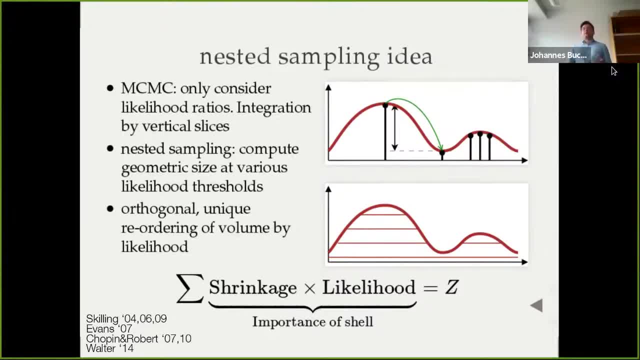 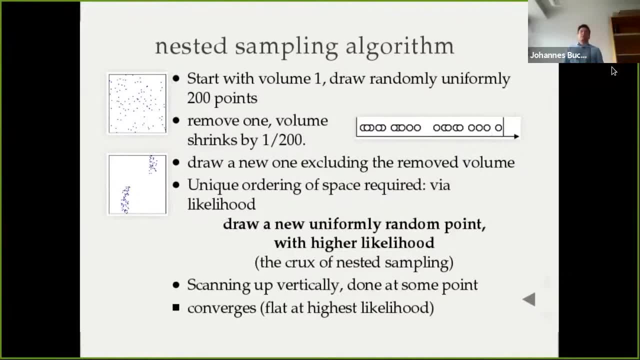 the evidence and the importance of each shell gives you the posterior probability distributions. So how does the algorithm work? Basically, imagine your parameter space is two dimensional, like shown here on the left. you throw in 200 points and you find the one that gives you the worst fit. 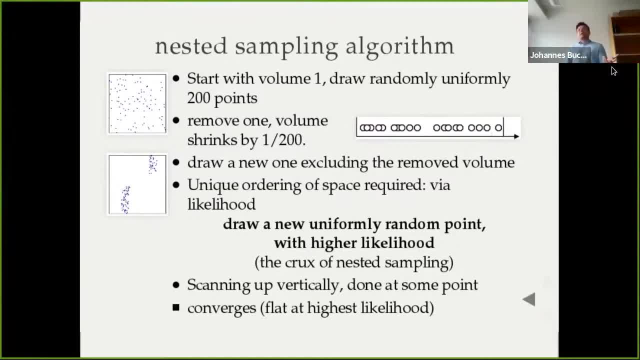 And you take that one out and you have to imagine the volume represented by these points that shrank by a factor of one over 200.. And now you put another point in, drawn again uniformly according to the prior distribution, but with the constraints that the fit has to be better. 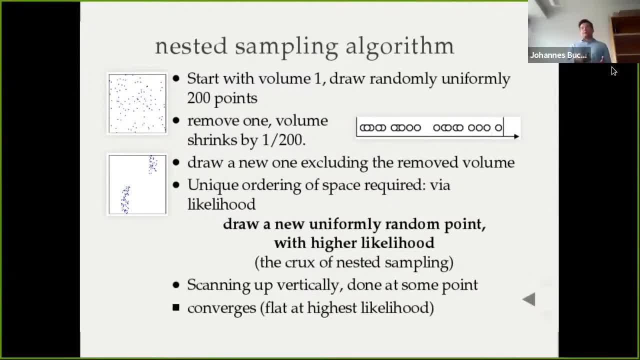 than the one you just took out. So, and if it doesn't, you repeat the process, And if you do this iteratively, in every iteration the volume shrinks by a constant factor one over 200.. So you are, we are keeping track. 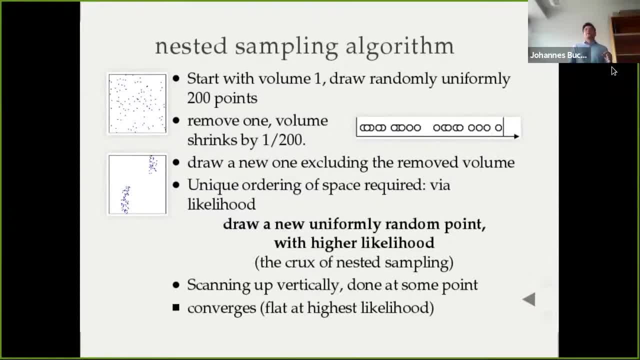 of the volume that is accessible, and you have access to the likelihood, the height of each of these slices, by the likelihood that you just removed, And if, as you iterate and iterate, you always take out the worst fit, And so you end up in a situation where all the points 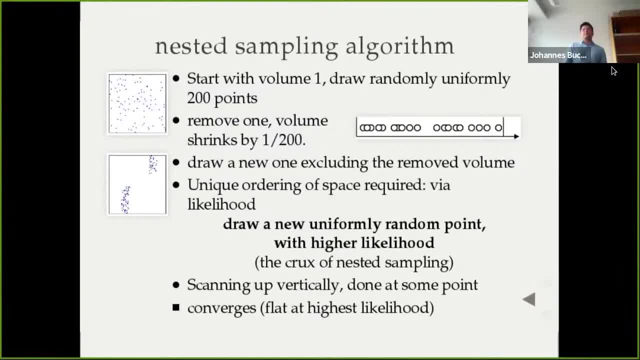 are concentrated at the best fit, or near the best fit, in a very tiny read volume, And then you can stop because you're into, that tiny volume doesn't contribute. It doesn't contribute to your integration anymore. Now the missing piece here is how to draw this unit. 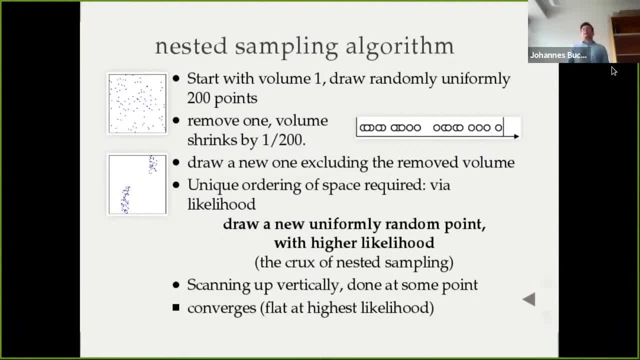 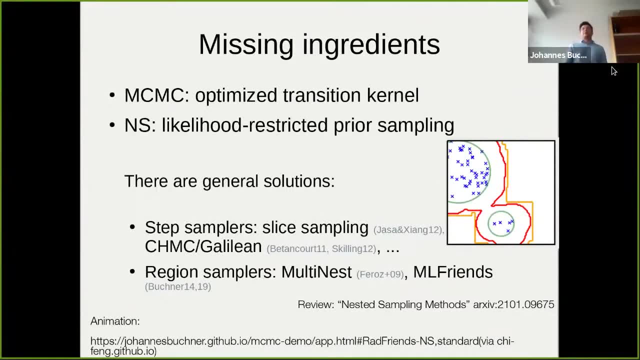 uniformly distributed random point. but with this likelihood threshold And just like in MCMC, you have to put in some transition kernel in nest sampling. You have to put in that that process for this likelihood restricted prior sampling. But the nice thing is about nest assembly is that there are 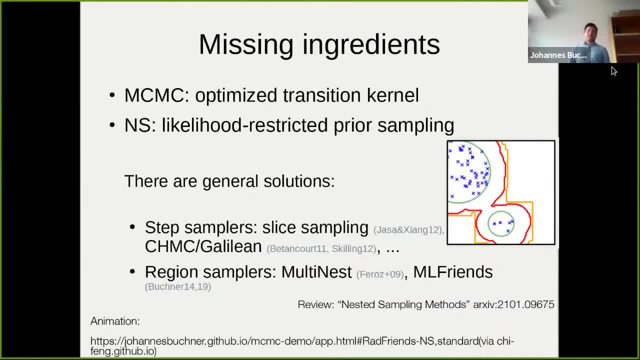 general solutions here. Basically there are two big classes, Some random walk algorithms And the class that I will talk about are those that use the existing points to find the neighborhood region and only sample from that neighborhood region. And quite famous is multi-nest, which clusters the existing points. 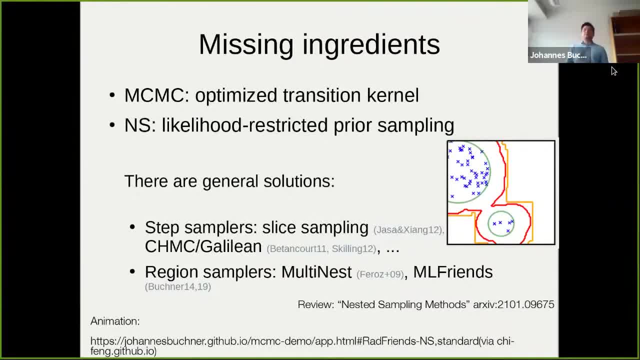 with the clustering algorithm into ellipsoids and uses some a bit more ad hoc criteria to say split these clusters. And I will mostly be talking about ML friends, which is another algorithm which doesn't use this kind of ad hoc clustering. 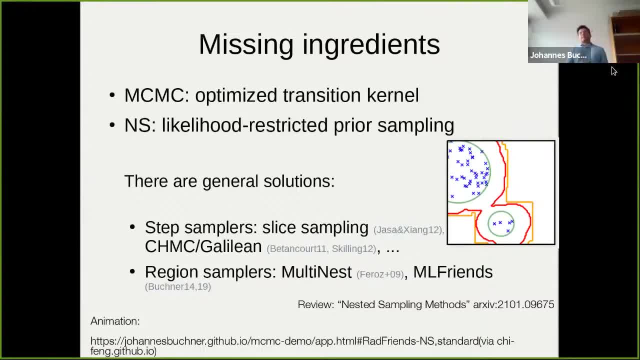 but builds ellipsoids around each point and then cross validates, leaving some points out to make sure that the region built is robust and you have some safety guarantees, And so this is a bit more well-motivated, less ad hoc algorithm to use as nested sampling. 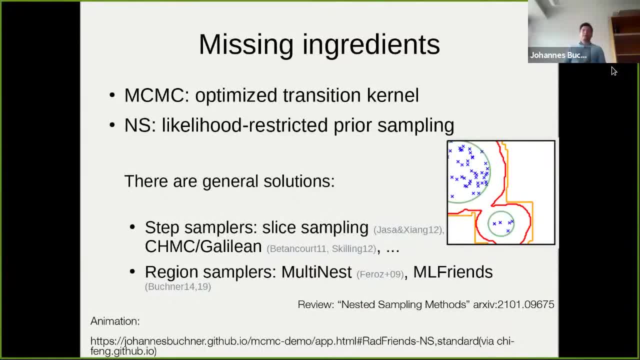 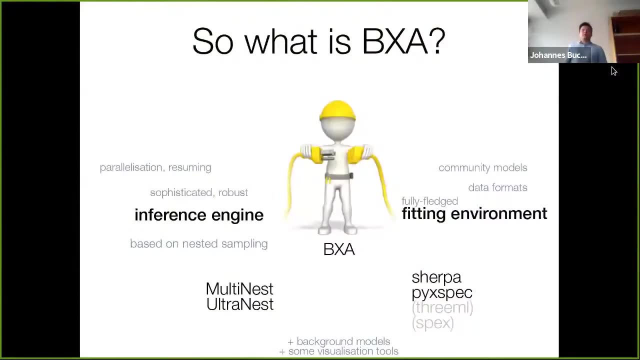 And it's. but both of these algorithms work really well in practice and give usable results with realistic models. There's a review and there's some animation that you can check out how the algorithm process progresses. But let me just come to BXA. 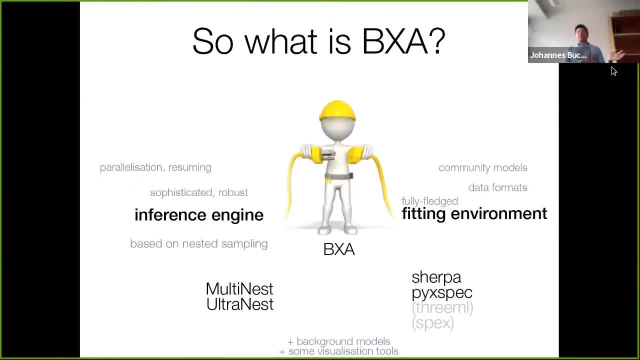 So what is BXA? Well, it connects one of these inference engines that is very robust, based on this sampling, with a full, with fledged fitting environment which has community developed legacy models and new models that come in and the established data formats. 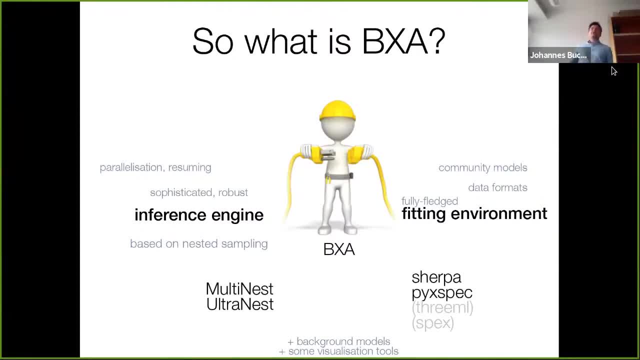 And you. for example, Sherpa and PyExpect can be connected with BXA to multi-nest or ultra-nest in the latest versions And that's just a hundred lines of code in essence. of course, now it does a little bit more like background. 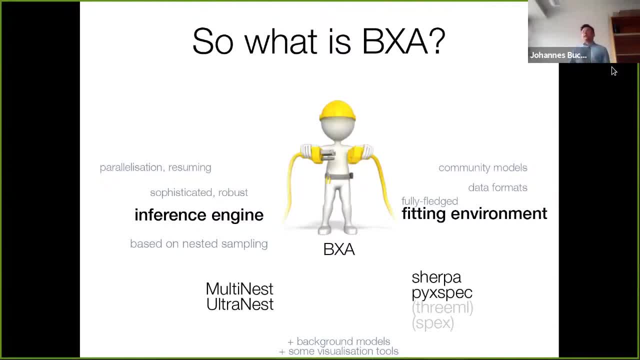 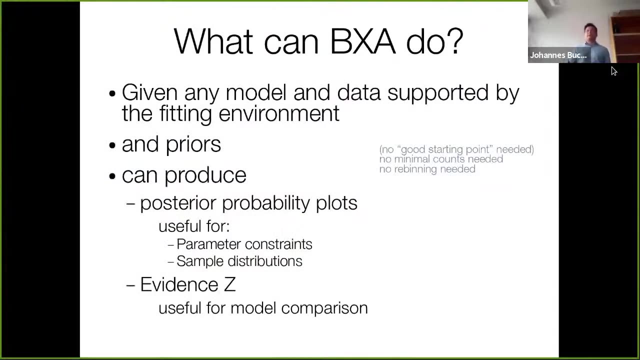 models and visualization tools. but the point is what is really enabled by this? And what is enabled is that you can do very sophisticated analysis and get very interesting results on the probability distributions, And I'll show you some examples. So basically you can fit any model and data supported. 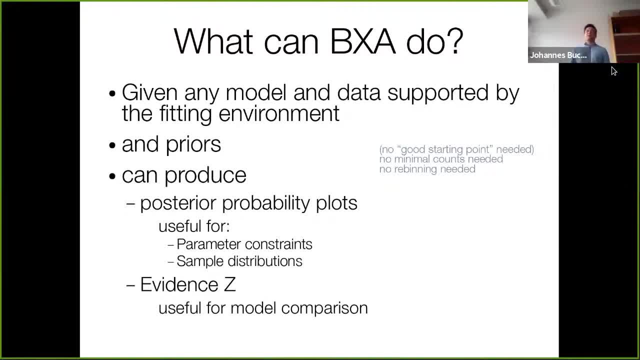 by whatever fitting environment you use. As long as you define the priors and you get posterior probabilities and the evidence for model comparison, You don't need to define a starting point, You don't need minimal number of counts And you don't need to weave in your data for that. 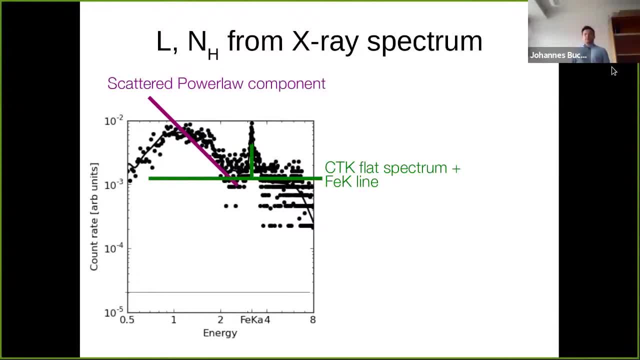 I'll just show an example here for the low data count case. So here I'm simulating a Chandra spectrum of a heavily obscured AGN. So it's an absorbed power law, some additional content scattering in green and an additional soft component in purple. 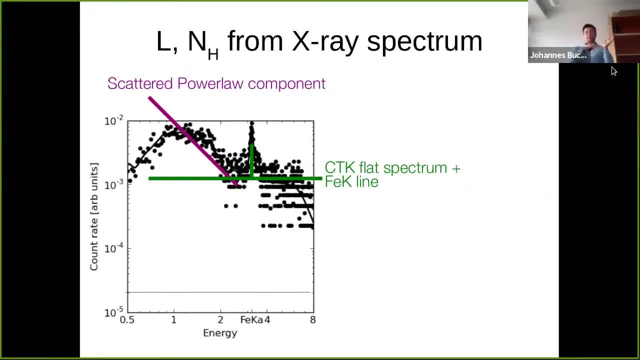 And what I'll do is I keep this spectrum shape the same as I used to generate, but I'll make it fainter and fainter, And on the right you will see the parameter constraints on the obscuration and luminosity. So initially, all of the probability. 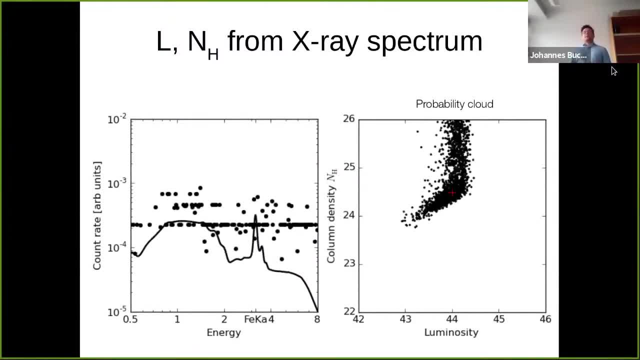 in the posterior samples is very well concentrated. but as you become fainter and fainter, lower and lower counts. this expands And at some point you even have two modes, two solutions here. But even if you have zero counts, you still learn something, mainly at the bottom right. 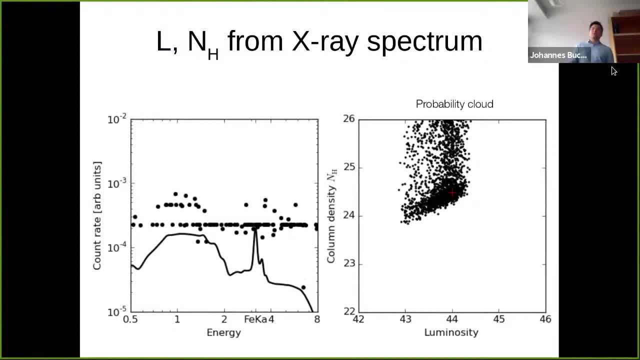 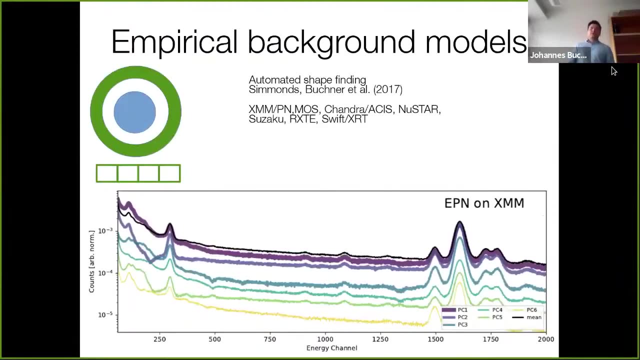 Quarter of this plot is always excluded because otherwise in the bottom right you would have a luminous, unobscured or less obscured AGN And that you can exclude already with your low count data. So there's no limits here. VXA also includes empirical background models for a wide 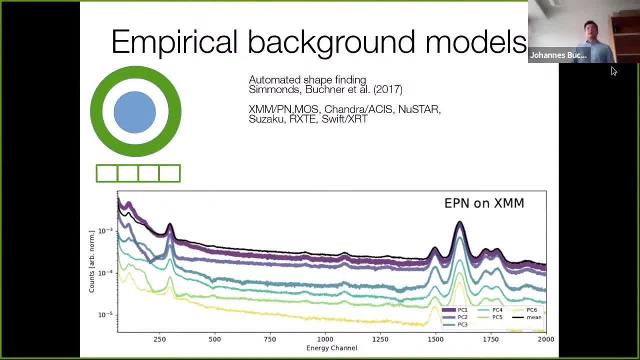 variety of missions shown here that we developed in Simmons, and all using a machine learning method. We basically did a PCA analysis on archival data and it's quite neat to use these because you get more signal to know it or you get more signal out because you put in. 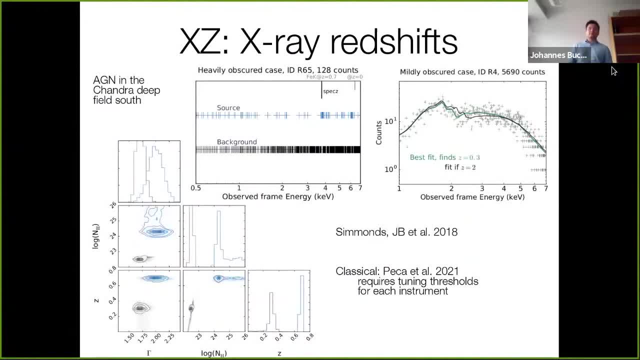 more information about what your background is supposed to be, And one example application here is X-ray redshift sweep. In the deepest Chandra observations in the Chandra Deep Field South, it's quite difficult to find the redshifts of active galactic nuclei because the exposures are so faint. 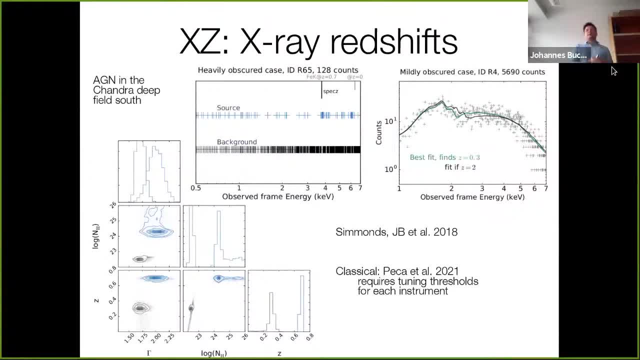 There are so many possible counterparts in these deep surveys that you could assign that source to, And furthermore it's difficult, even if you find the right counterpart. it's difficult to get optical spectroscopy to measure the redshift, So it would be neat to get those out of the X-rays directly. 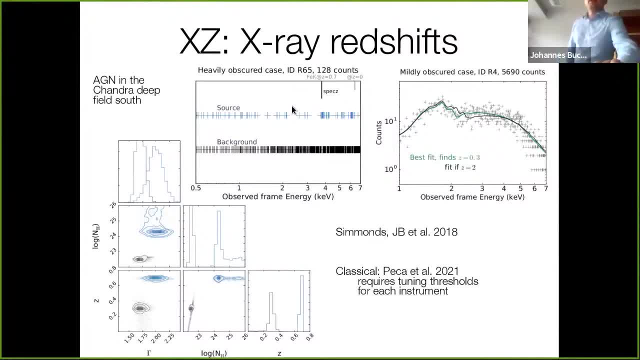 And what you'll see, what you see here in this plot is the source spectrum and you see a bit of a clump here which actually corresponds to the RNK line at a redshift of 0.7.. And on the right you see a less obscured case. 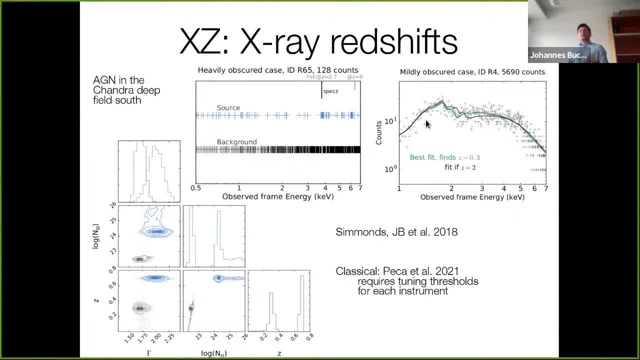 so not a complicated AGM like on the left, a less obscured case, and you see some wiggles here, but it's very difficult to tell by eye what is instrumental wiggles and what is. what is absorption edges that you could 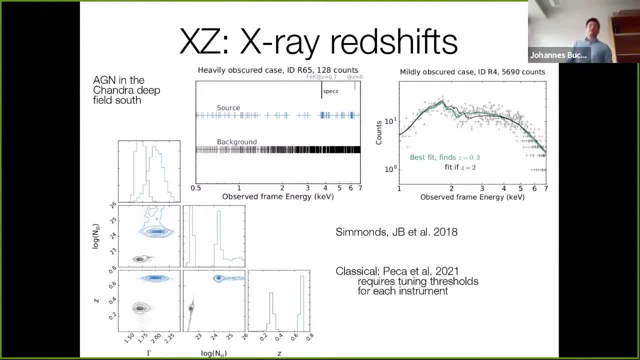 also use for redshift. But if you put all of this into BXA and use a sensible X-ray obscure model, you get the posterior distributions here on the left And indeed you can constrain the redshifts to the true spectroscopic values. 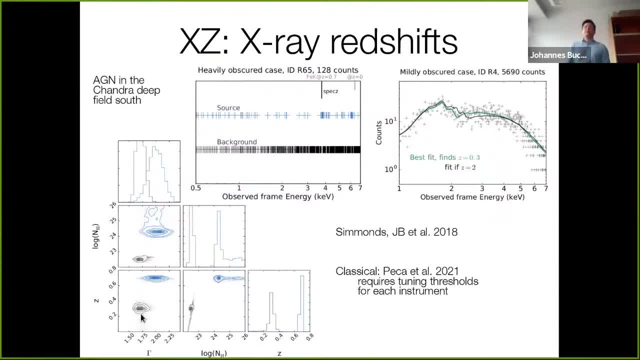 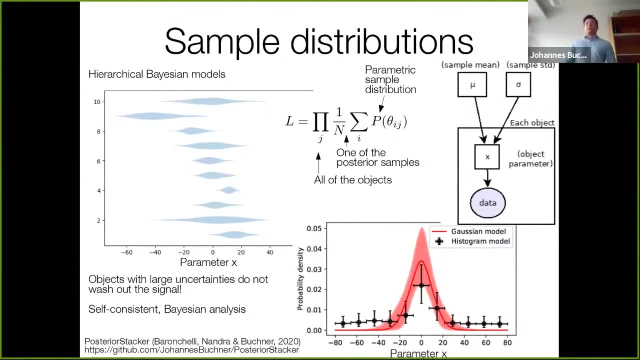 And here in the Bayesian inference, I didn't have to do anything specific about each instrument, Whereas in the classical analysis you would have to tune thresholds for each particular instrument you analyze. Once you have these posterior distributions, you might want to go further to sample distributions. 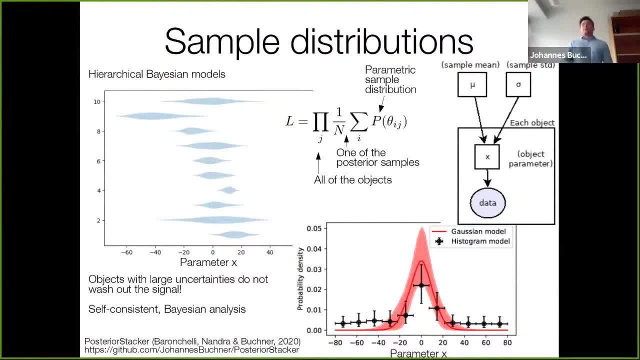 For example, here on the left, you have some parameter and at each epoch of your object, or or many objects, you have these probability distributions And you want to infer what is the intrinsic distribution incorporating all these uncertainties. And there is a very neat technique to do that. 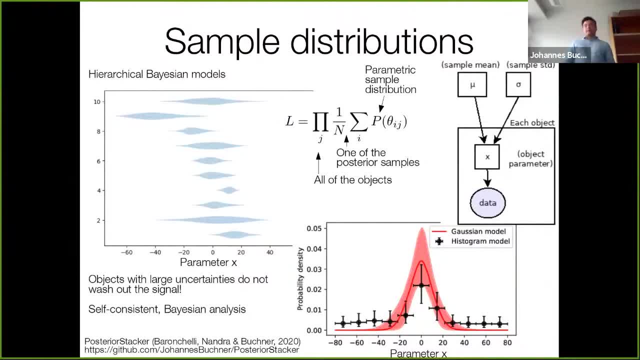 I think there's a lightning talk on that, called hierarchical Bayesian models, And the neat thing about it is it adding additional, less constrained objects doesn't wash out your signal And it incorporates all that uncertainty And we have an implementation called posterior stacker. 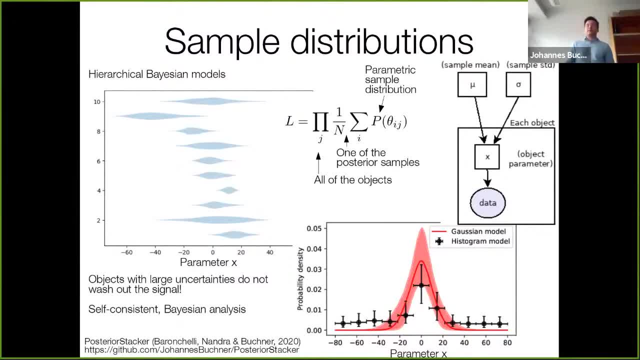 that does this and produces plots like on the bottom right. here you get the intrinsic or the sample distribution out, and it can ingest outputs from BXA And so it can then send out data for whatever analysis you MCMC or whatever analysis you've done before. 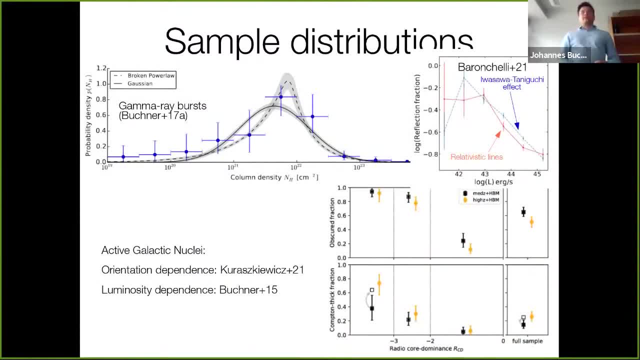 And here is show some examples. on the top left you have gamma reversed obscuration distributions with column density, fitted with a couple of sample distributions like the Gaussian. If you just look at the mean of this Gaussian, you could also divide these kinds of samples up. 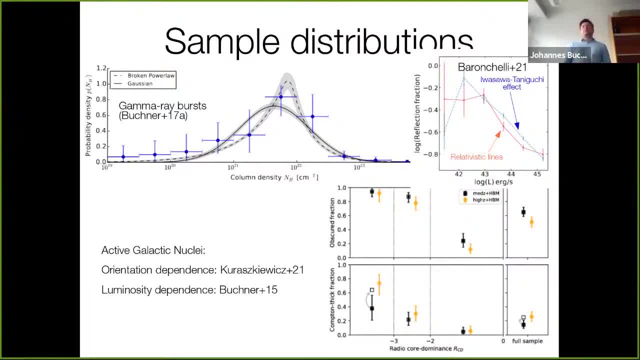 and look how the mean behaves in these different sub-samples. And this is what Barancelli et al did on the top right here for the reflection in sort of intensity, for the narrow in blue and in red for the broad relativistic lines. 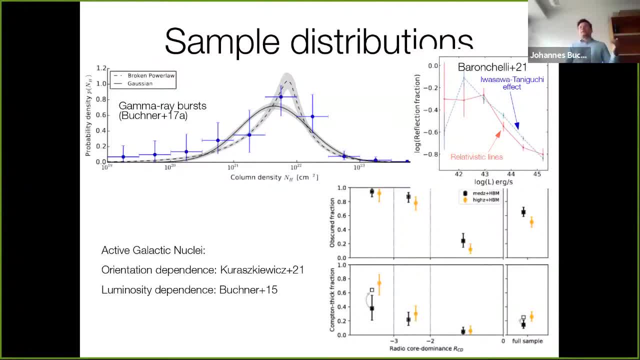 And what Barancelli found here is that for both there seems to be an effect of luminosity. On the bottom right is a similar analysis for the obscuration fraction as a function of orientation of the AGM. So very interesting analysis you can do here. 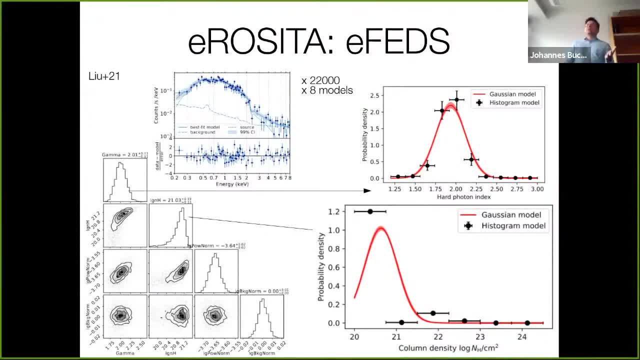 I want to also highlight Eerozita, where recently we've released the effects field with 22,000 AGM in there, which we've analyzed with eight models. So you can imagine the computational complexity and you really need a good inference machine that can deal with this. 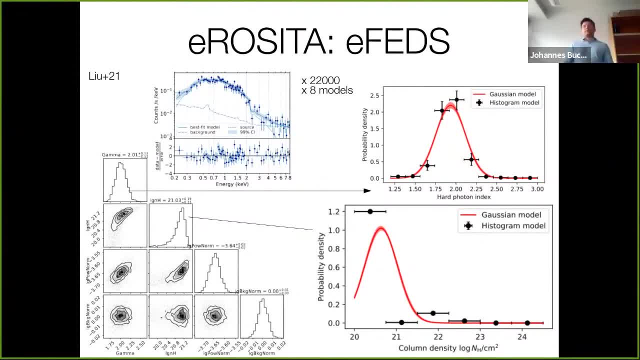 So we have the X-ray system, we have the X-ray spectra in blue here, get probability distribution for each model And then you want to do sample distributions like shown here on the bottom right. You get the column density distribution of that particular sample and the front limits distribution top right. 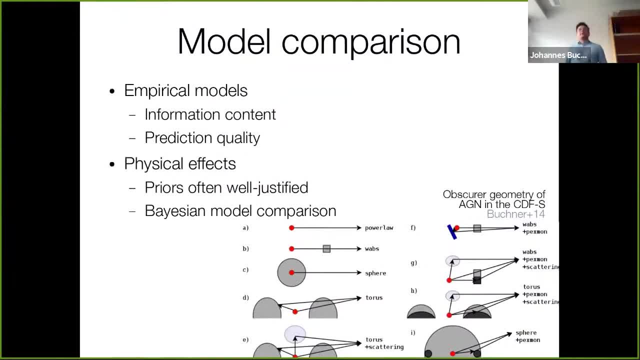 Now I want to talk a bit about model comparison. For model comparison, it's always important to keep in mind what question you're asking. So if you have, for example, just empirical models that try to approximate the shape or the effective behavior of your data, 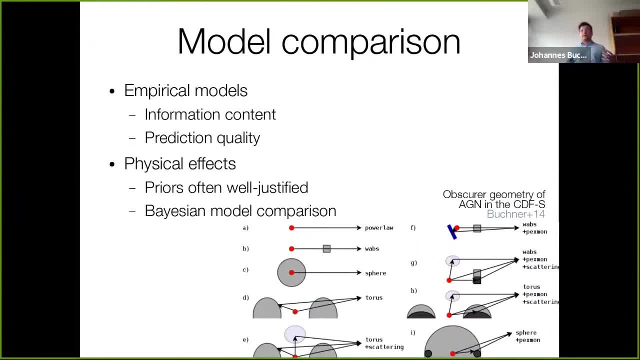 then you might want to just look for the model that has enough capability to store the information contained in your data. So you want to do something information theory-based, or you might want to pick a model based on how well it extrapolates to data it hasn't seen. 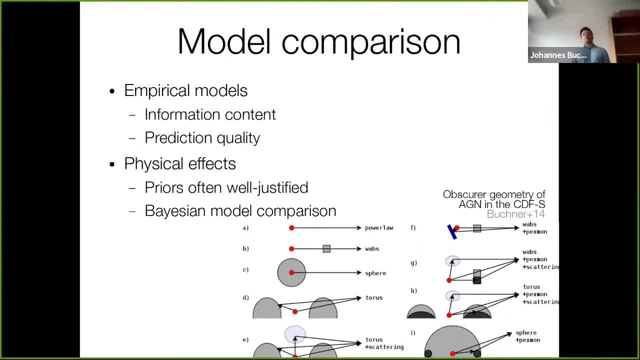 That's very common in machine learning sort of prediction quality. But if you have models that are that differ in the physical scenarios, often in these cases have a well-justified priors for all of your parameters and you can do Bayesian model comparison with the evidence and base factors. 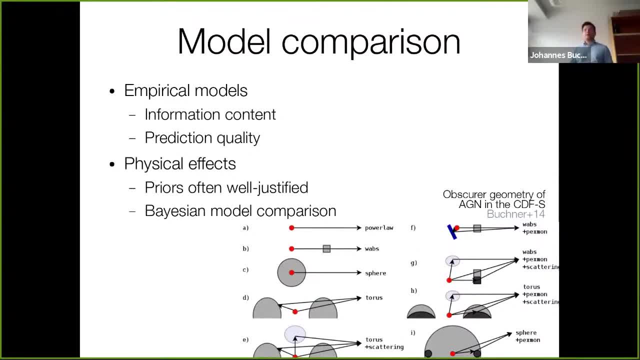 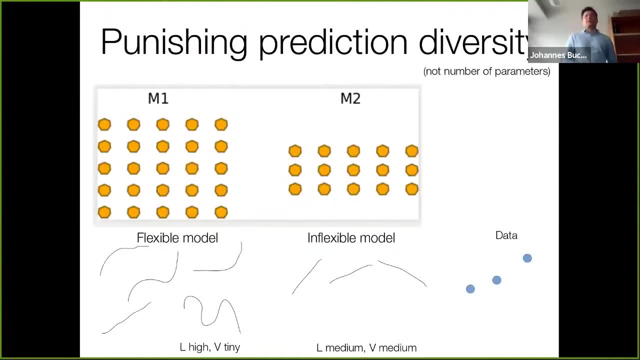 And that's what we did in 2014. on the bottom right I show different obscure geometries that are plausible and we were able to distinguish between these different physical scenarios using model. And just to illustrate how that works, Let's say you have one model that is relatively inflexible. 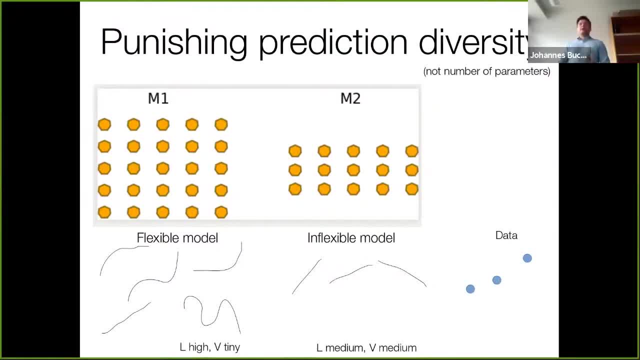 like illustrated in the middle here, and two can just make some more of those line shapes and it sort of fits your data reasonably well, but in some region of its parameter space. But if you completely include also another model which is much more flexible, like the one here, 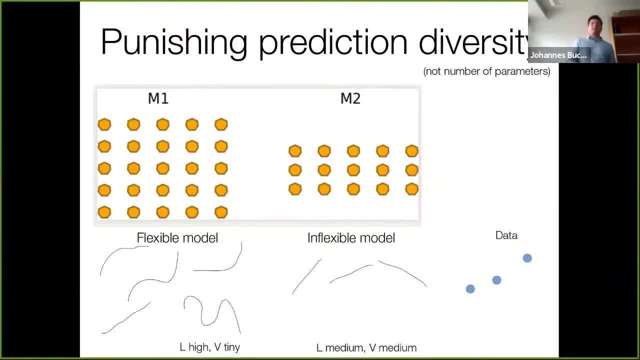 on the left So you can make all kinds of twisted shapes. Then you will of course find a better fit, higher likelihood, but it will be in a very small volume of this parameter space, Because as soon as you move away, the model has to do something very different. 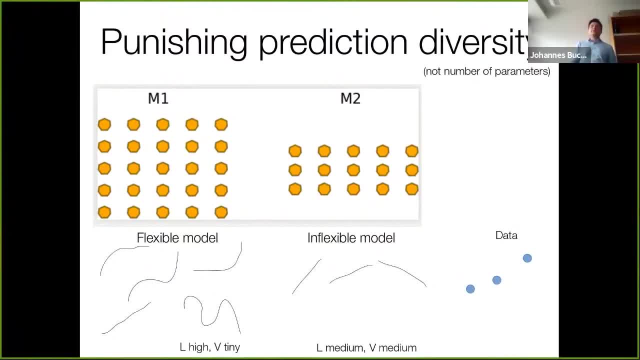 because it's very flexible and will make a different shape, And so the multiplication of likelihood and volume will be lower because the volume is so small. And, in other words, this prediction diversity, this unused prediction capability is being punished by this averaged likelihood. 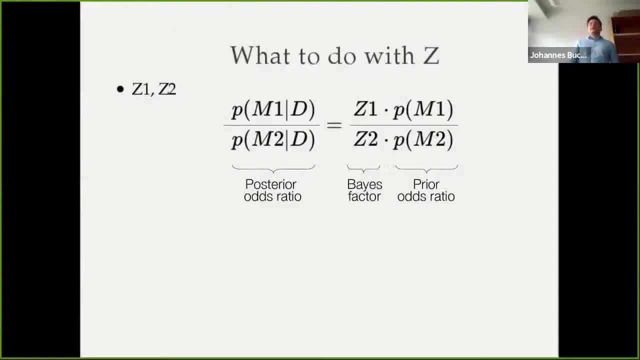 marginal likelihood, And so you can do this. integral ratios Z1 over Z2. here is the base factor. If you multiply that by a model prior odds ratio, you get a posterior odds ratio which tells you the probability of model one compared to probability of model two. 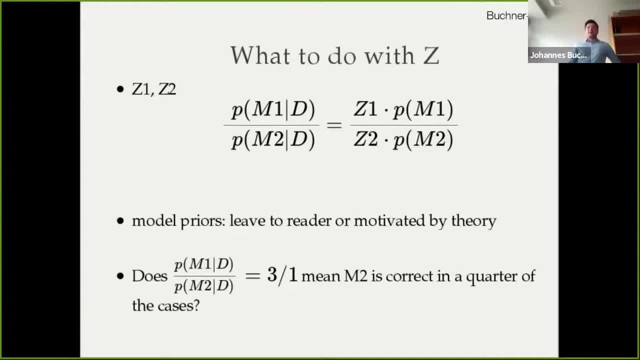 The drawbacks here are that you need these model priors. Either you have a good idea for them. And the second issue is: just because one model has a higher evidence value, that doesn't, and you decide to say, okay, this is my true model, I'm going to pick that one. 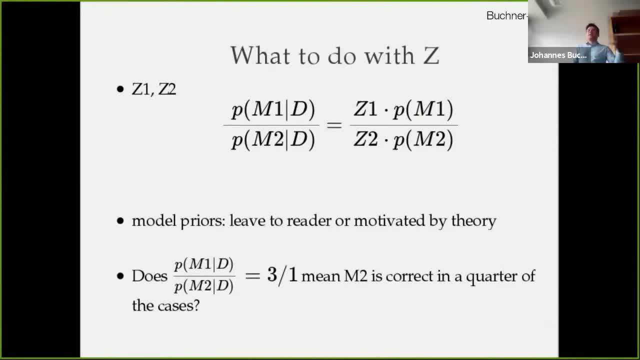 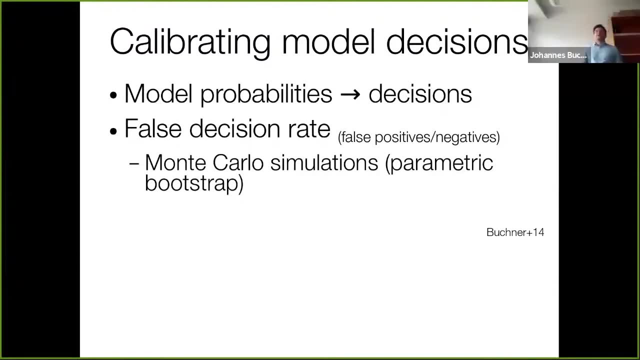 It doesn't tell you the ratio, the rate at which you would make a false decision. So what I would? yeah, So what I would recommend is to always make simulations. So generate a bunch of data on one model and on the other model and you try out. 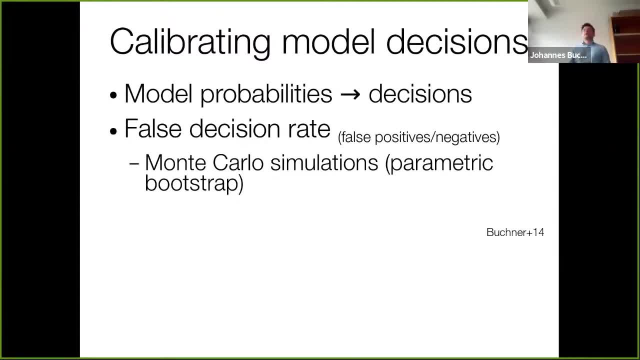 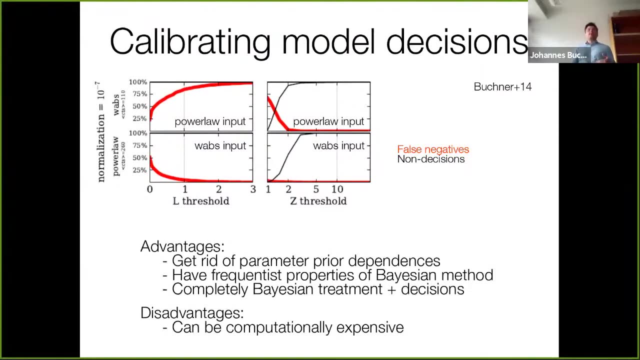 how often you would make a false decision. So that allows you to get base factor thresholds, And the nice thing about this is then you have the best of both worlds. So, basically so, here's an example from one paper where we also showed that this works better than likelihood ratios. 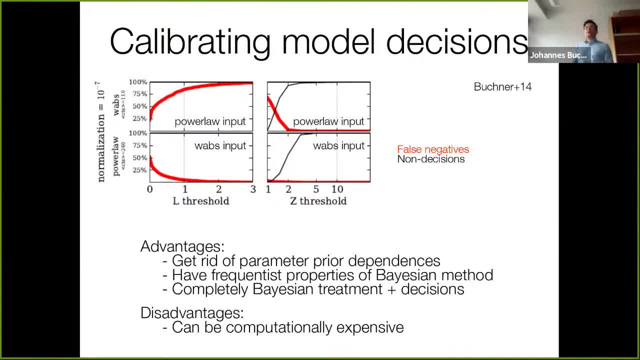 The advantages here is you get rid of the parameter prior dependencies. You have these frequentist properties on some Bayesian methods, so you know how often it would be wrong, but you still retain this interpretability of the base factors and the consistent Bayesian application. The disadvantages: is computationally expensive. 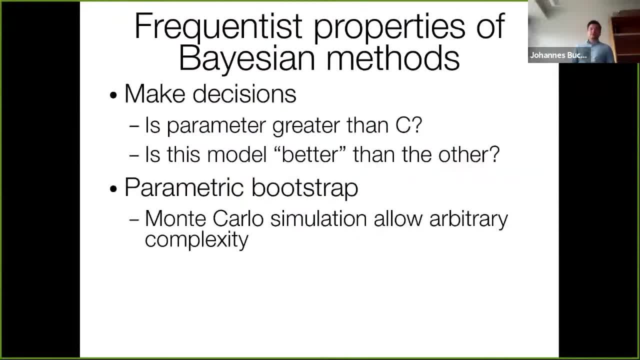 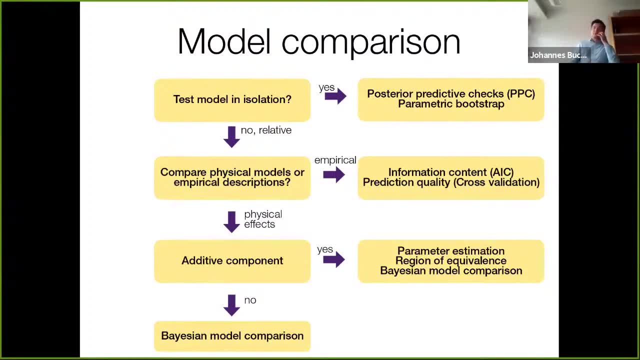 but with nested sampling it's actually feasible. I think I said that. So yeah, there are a couple of styles to do model comparison. If you just want to test the model in isolation, you probably want to do posterior predictive checks or parameter bootstrap. 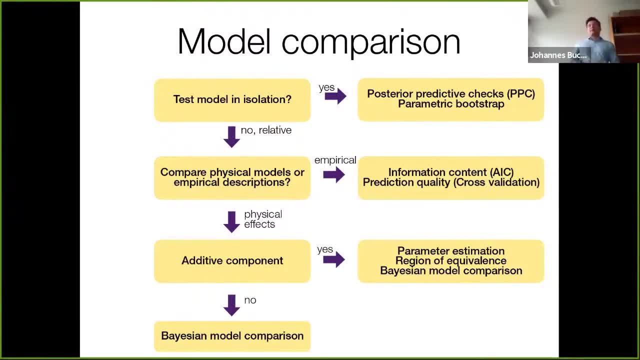 If you have competing models, it depends whether, as I said, whether they're empirical or whether they are more physically motivated, If they are nested. if you have additive components- maybe you just want to estimate the model- you can estimate the strength of that additional component. 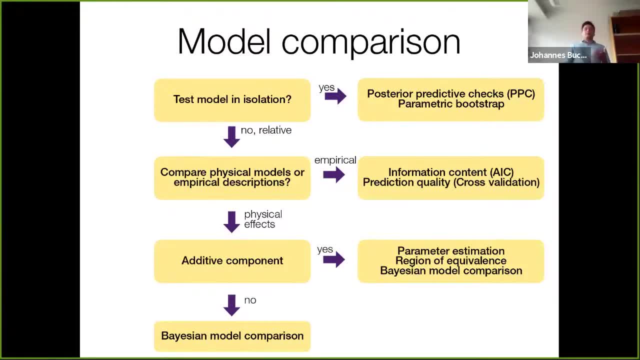 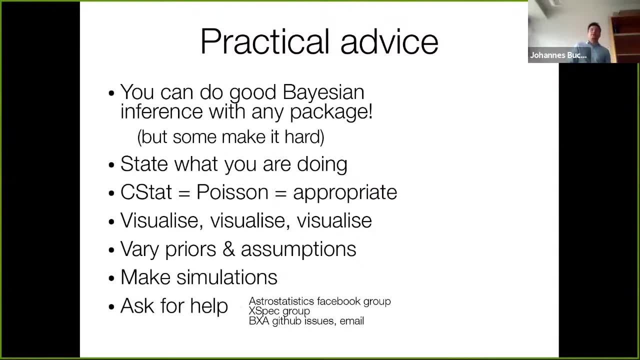 and you can just do parameter estimation or you can do a Bayesian model comparison. So just so, I will just finish with some practical advice. You can do a good Bayesian inference with any package. Some make it easier than others. It's important to state what you're doing.